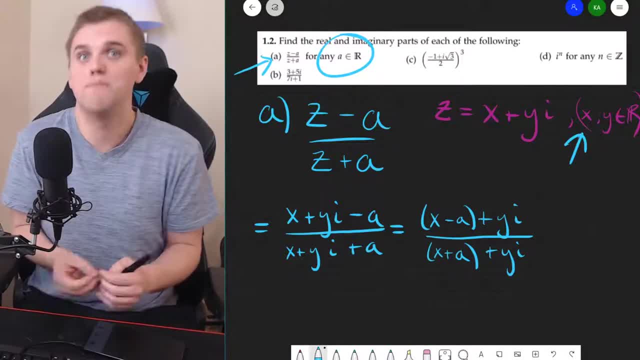 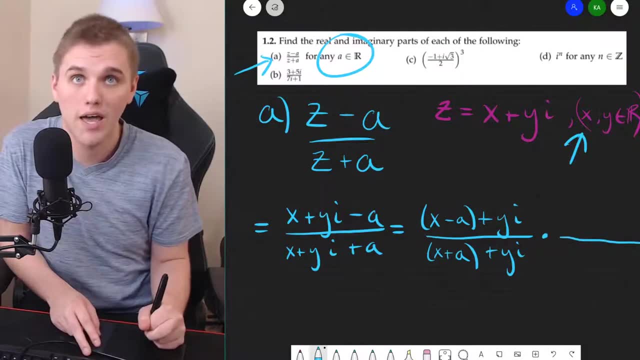 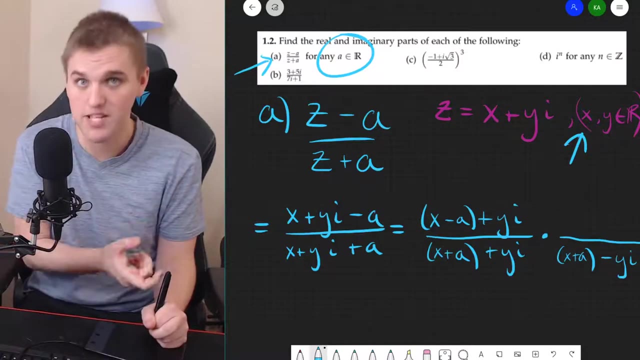 And the way you do that is, you multiply your denominators by the complex conjugate. And so I'm going to multiply the denominator here by the complex conjugate, which is x plus a minus yi. I flip the sign of the imaginary part. 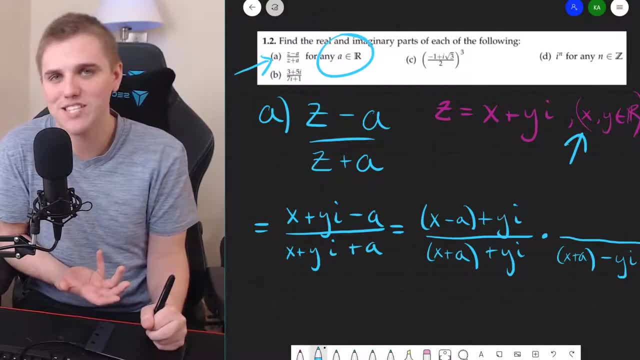 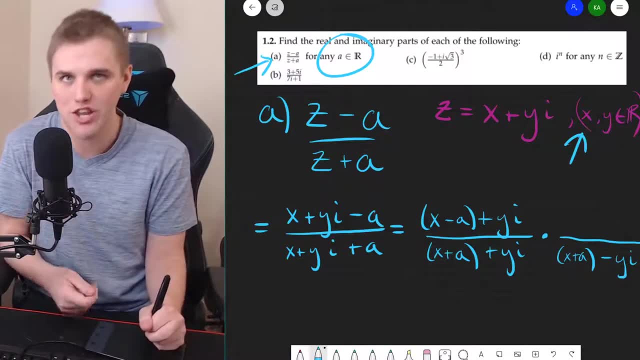 Now I can't just multiply by whatever number I want, because that will probably change the number. So I need to make sure I multiply by 1, because multiplying by 1 doesn't actually change the number. So I need to make sure my numerator here is also the same. 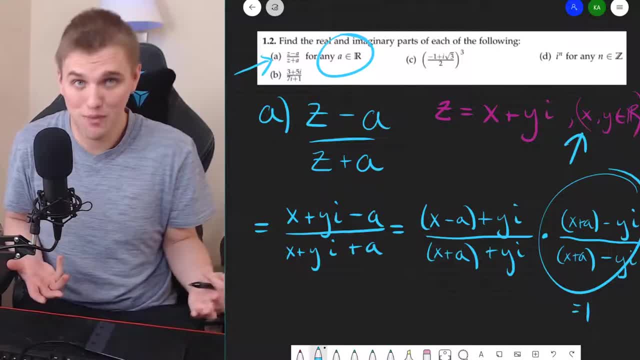 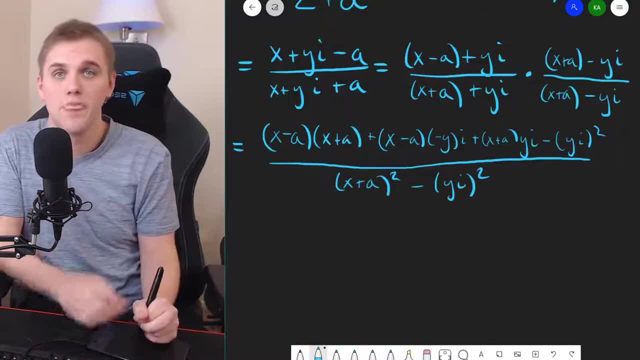 That way, this whole number right here just equals 1.. And so I'm just multiplying by 1.. Alright, so let's expand this out. It's going to get a little messy, but just bear in mind you're going to have to do it at some point. 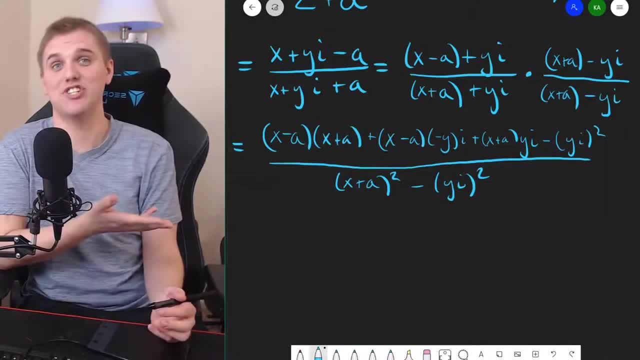 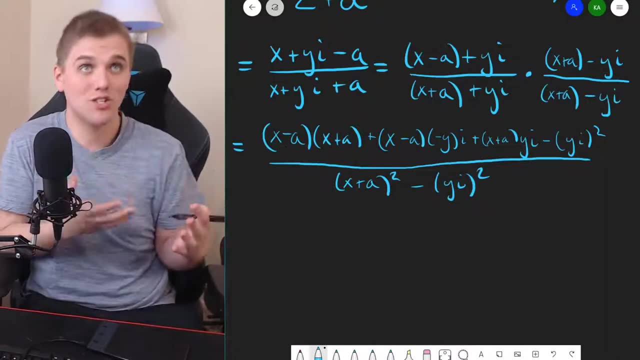 So, like I said, this is one messy multiplication. This looks gross but it does simplify a little bit. Let's try to combine like terms and simplify. We can also FOIL and expand some terms, So let's do all that. 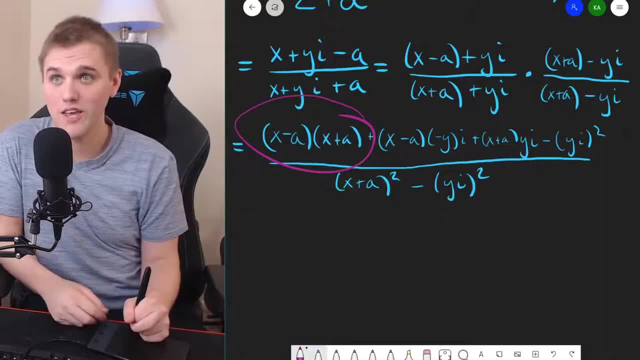 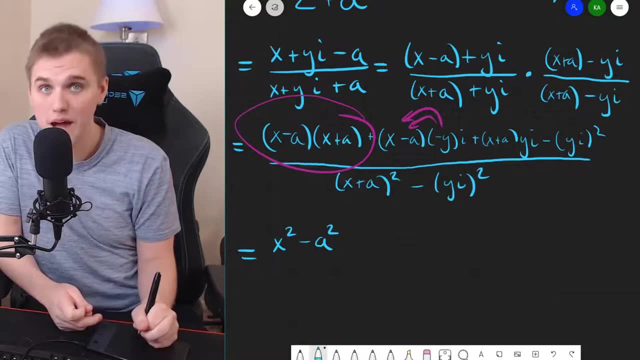 The first thing I'm going to do is I'm going to multiply these two terms by FOILing, And then I'll do the same for negative y here, Keep in mind that there is an i right here that I have to keep in both terms. 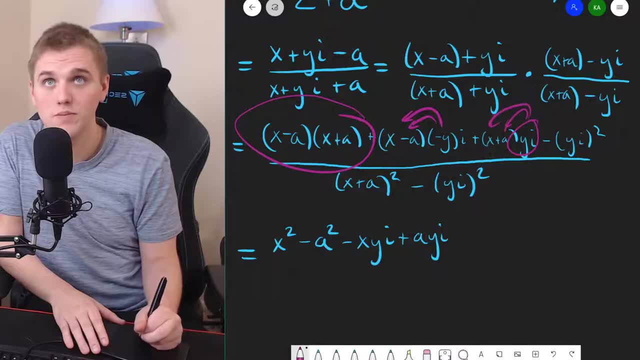 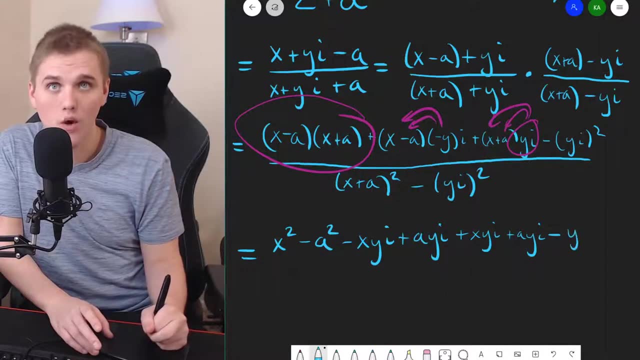 I'll do the same thing with this yi in both of these terms. And then, last but not least, yi squared is just y squared, i squared, but i squared is negative 1, and so the negatives make a positive. Okay, so still looks messy, but again we can clean things up. 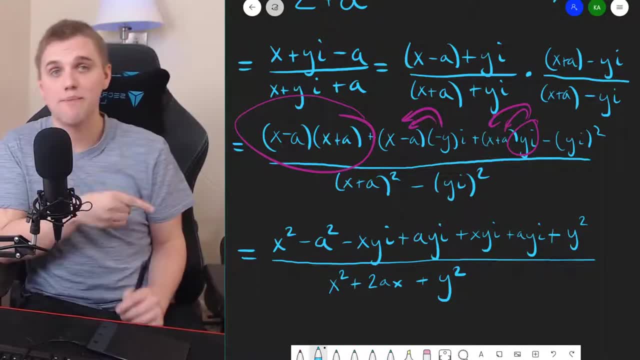 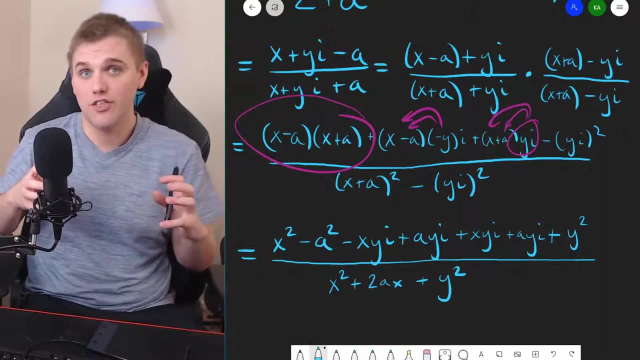 The way we're going to clean this up is I'm going to separate this fraction into two different fractions. Specifically, I'm going to group together the terms that are real and I'm going to group the terms that are purely accurate, The imaginary, together. 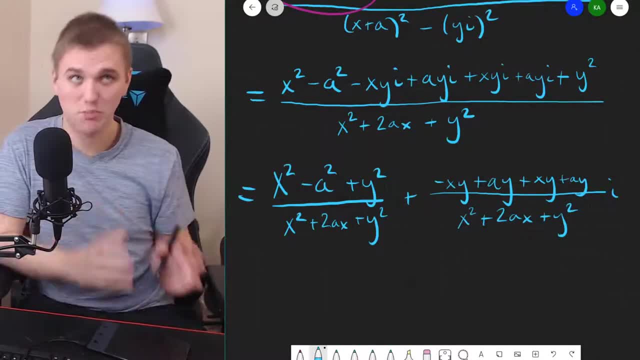 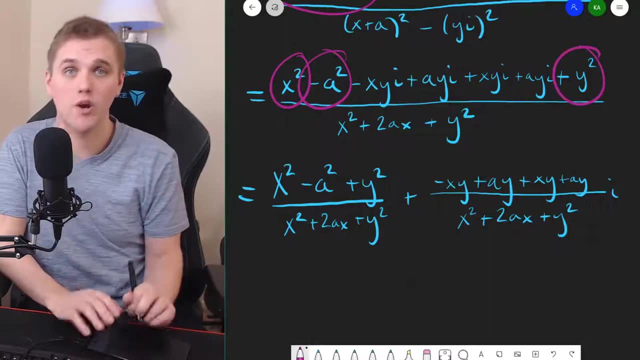 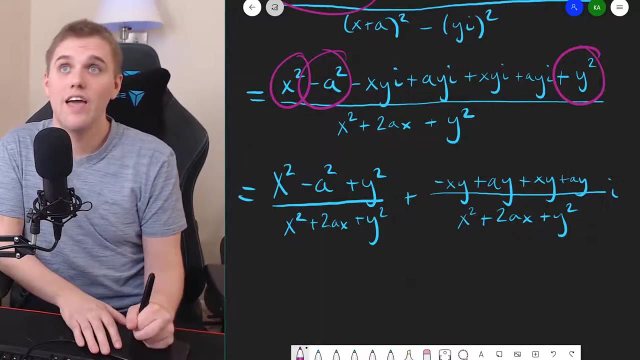 Okay, so I split up my fractions and simplified a bit, So let me explain what I did. So first I grouped together my real terms: My x squared minus a squared plus y squared. Those are all strictly real numbers. There are no imaginary components to either of those. 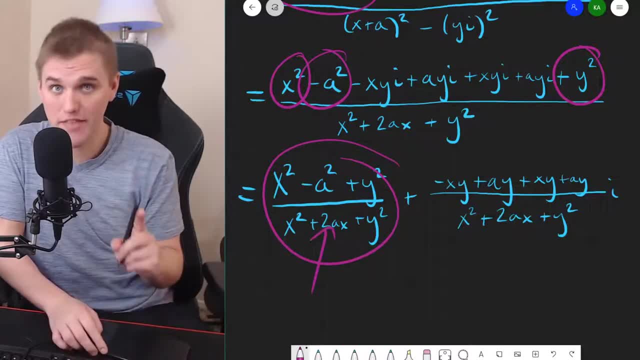 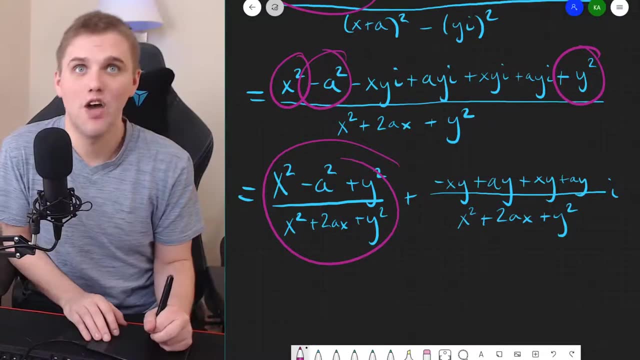 And that's how I got my first fraction here with this denominator, which I'll talk about that denominator, in a moment. And then my second fraction is just the rest of the fraction. Now notice here that none of these terms have an i. 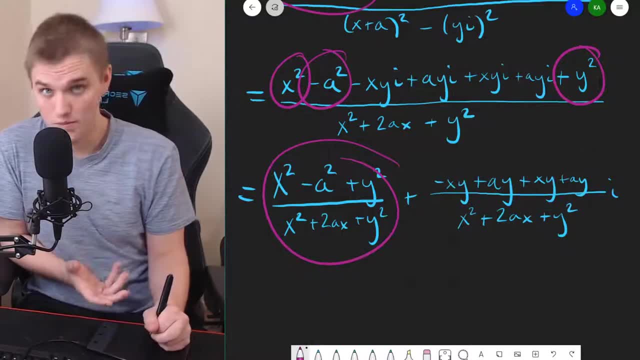 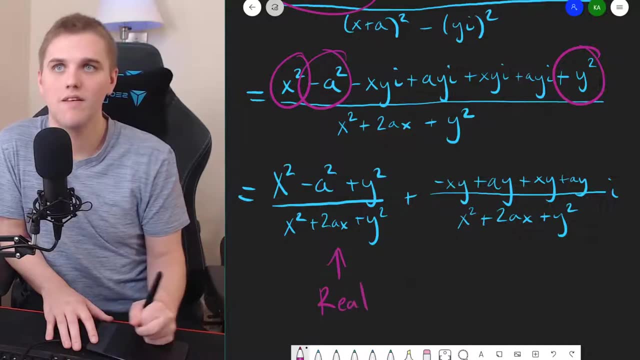 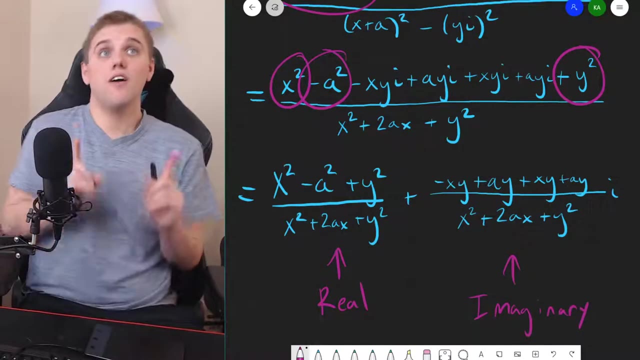 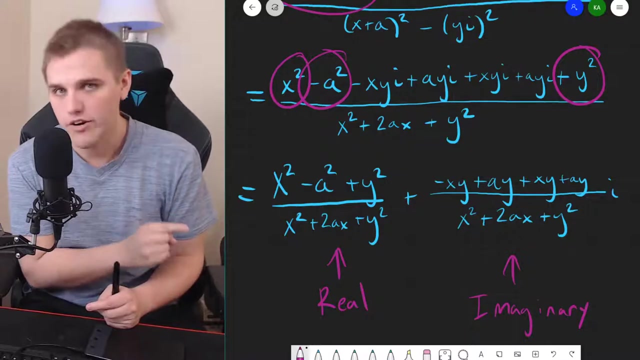 and that's because I factored out the i, to make it very clear that I have my real component and my imaginary component. Now a couple things I want to mention here: The denominator: How do I know that denominator is a real number? 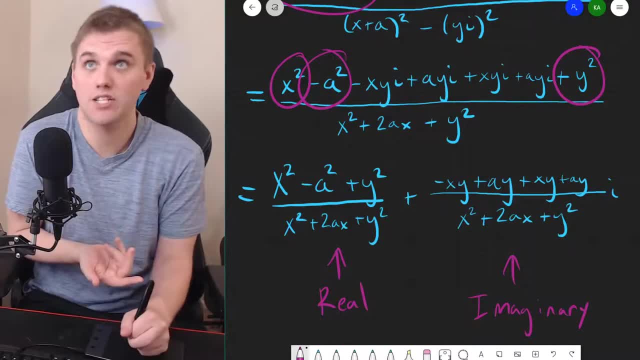 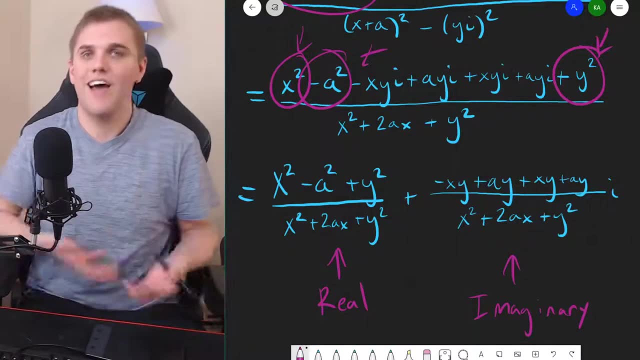 Like I know, the numerator is a real number because I specifically picked the real numbers in my numerator here. But if that denominator has a complex number or an imaginary part, then I haven't split up my number into its real and imaginary part yet. 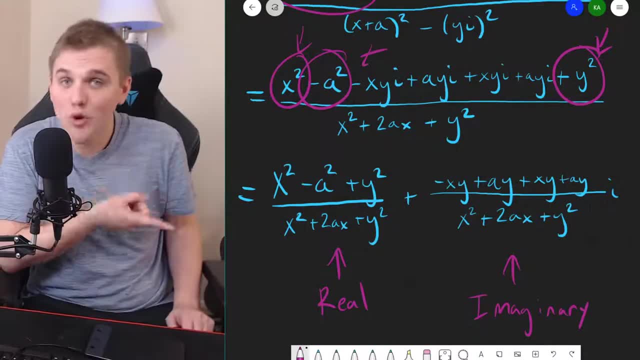 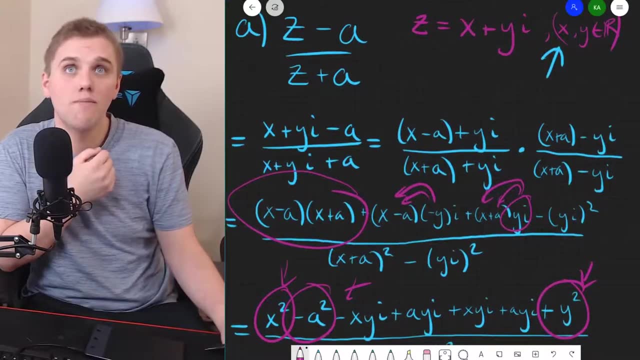 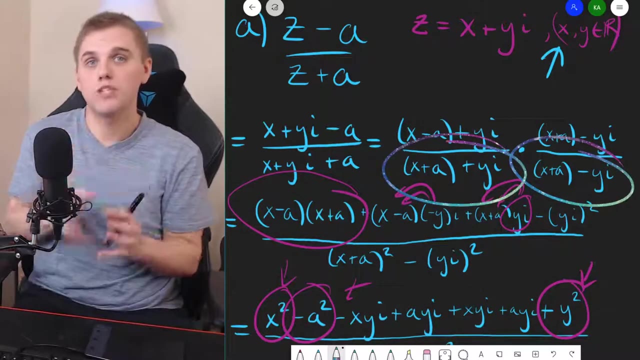 And so how do I know that denominator is a real number too? Well, that's because by construction in the beginning we multiplied right here by the complex conjugate. And when you multiply a complex number by its complex conjugate, 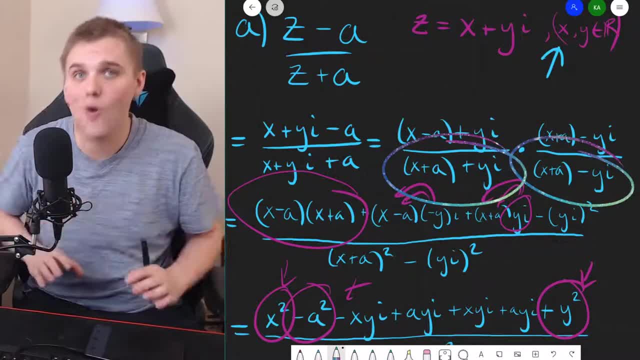 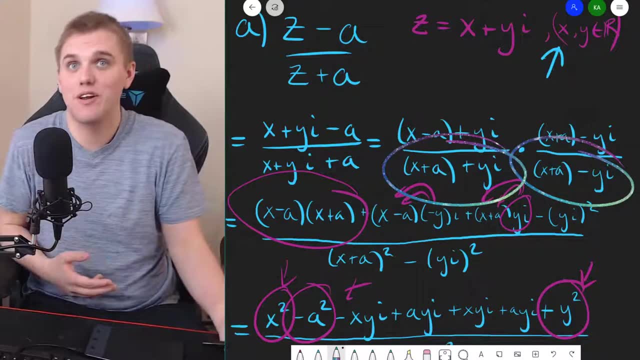 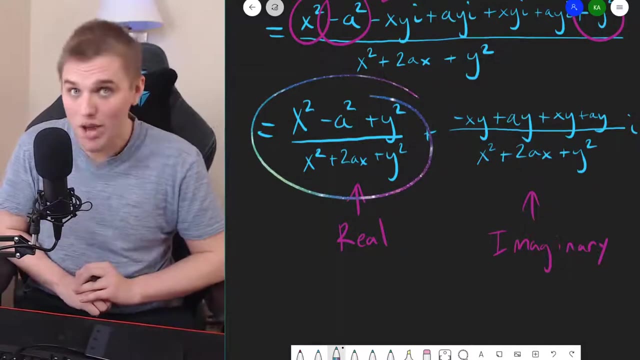 the output will always, always, always be a real number, And so, because of that, my denominator is a real number and my numerator is a real number, and so this whole term here is a real number. How do I know that? that's my imaginary part. 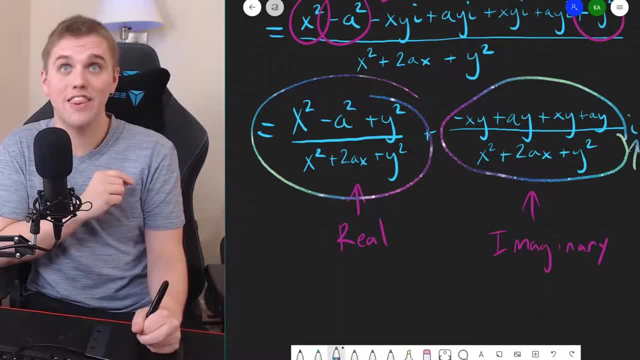 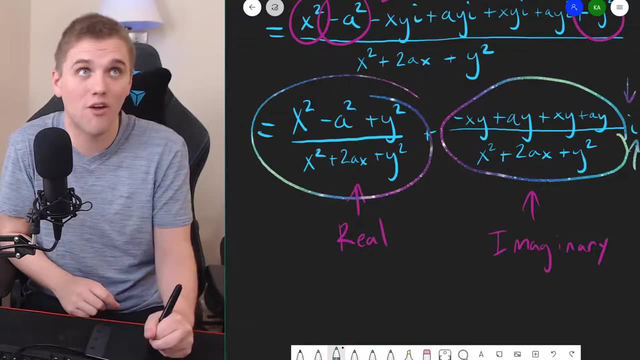 Well, we have to first make sure that the denominator is a real number, so that what's in the circle doesn't include an imaginary part, because the whole point of pulling out this eye right here on the right is so that I don't have any eyes in the imaginary part or the real part. 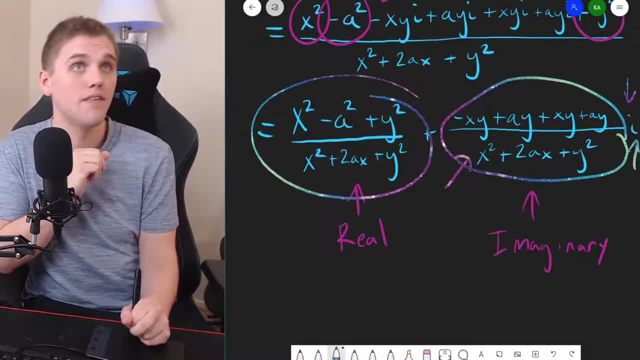 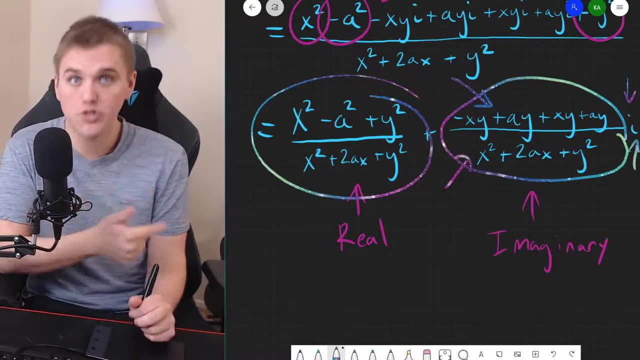 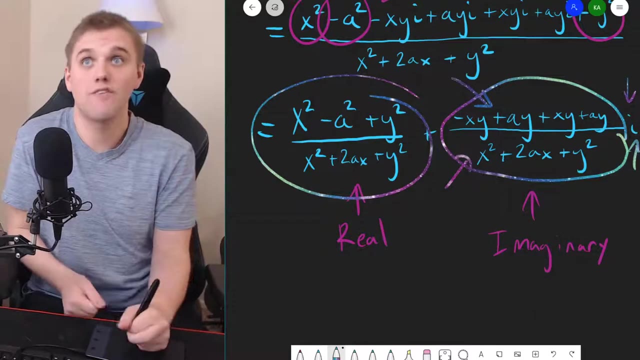 But again the denominator is the same, and this numerator is strictly the multiplication and addition of real numbers, which by itself is a real number, And so both of these fractions are real numbers, And so I have a real number plus a real number times i.